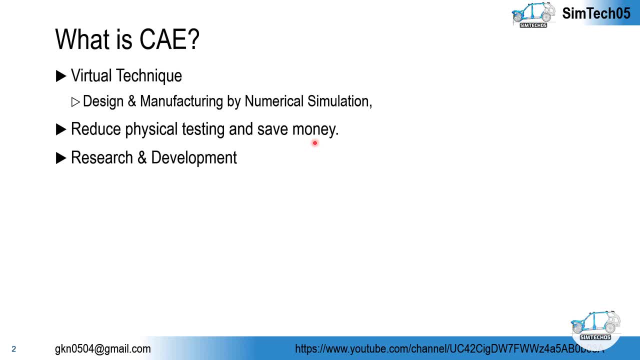 it's a virtual technique. Why we are seeing here virtual? Because even before phenomena or process take place we can check it virtually within the computer. So it's a virtually adapted software that can validate our design, can validate our manufacturing components with the 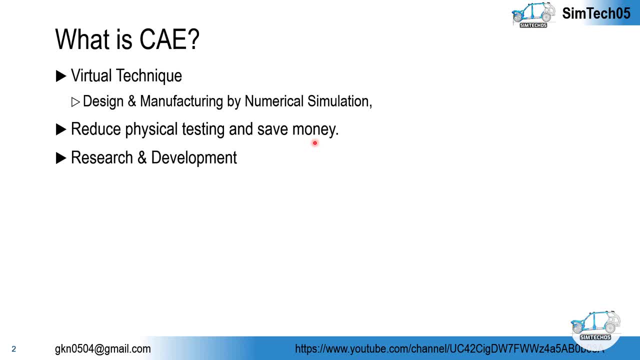 help of the simulation technique, with the help of numerical techniques. I'm not going to waste your time much in these theoretical sections. You know it very well. Like we can reduce the physical testing, we can save our money And it is the most important tool for the research and development. 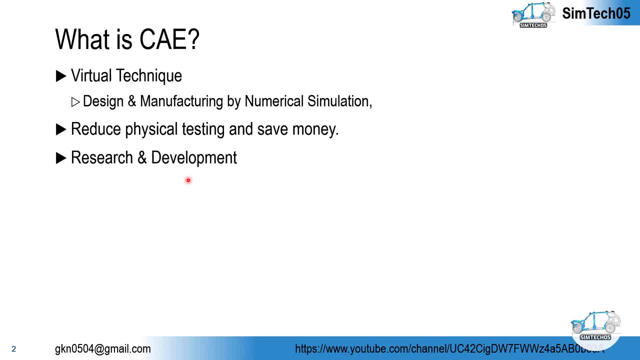 program or research and development department. Why? Because before even manufacturing the component, before even the process take place, we can check it And if we found any error or our design or assembly not meet the criteria, then we can modify within the development stage itself. That's okay. 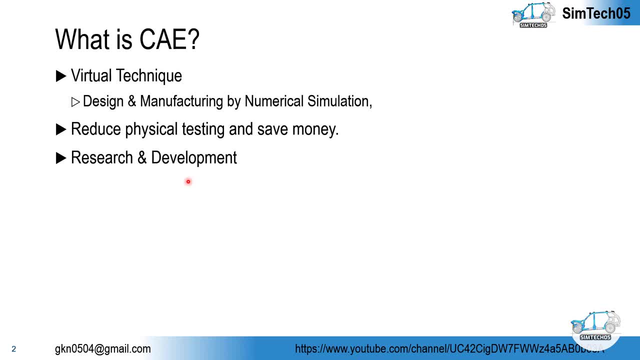 That's a theoretical portion. Now come to the original concept of this CAE. Yeah, of course, the CAE. we will gain a lot of progress there. We will make some modifications. Now come to the original concept of the CAE. here, of course, the CAE we need to solve. 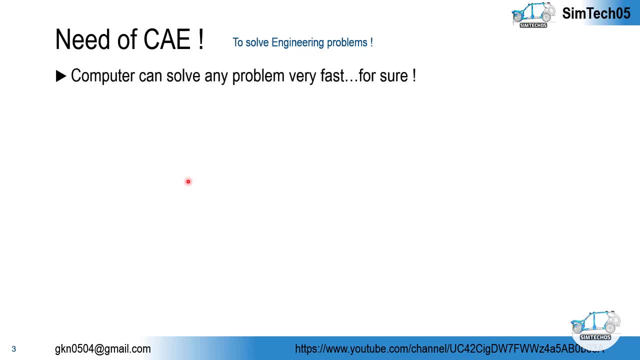 engineering problem with the help of numerical techniques. See, we have computers and the good thing about the computers: they can solve any problem very fast. but these computers have one problem. what is that problem? they can solve only things within the binary language, means computer can understand only the binary language. but in our real life, the problems 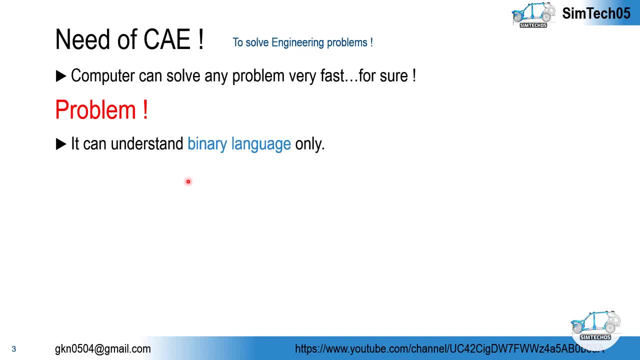 are not in the binary language. somehow we have problems. we can formulate the problem with the help of ordinary differential equation or partial differential equation or maybe some simple algebraic equation forms, but these equations computer cannot read directly. so do we have some options, some way, some method to convert those differential equations into binary? 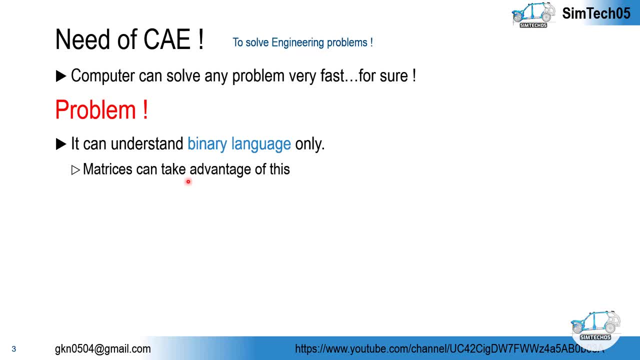 language. and can we take advantage? yes, we can take advantage of computer with the help of matrix. here we have one example: the stiffness of any object, any component, can be given in terms of matrix, and this stiffness may be function of material, may be structures, size and shape. so how we can do such conversion, that is the major point here. 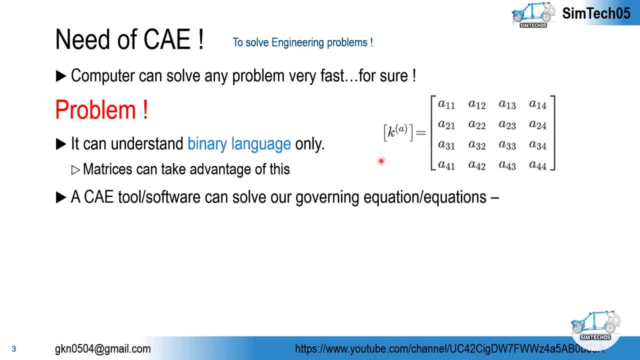 because once we convert our governing equation in form of matrices, then our CAE tool, with the help of computer, can solve our governing equations very easily. and in mathematics these governing equation may look like m x, double dot plus Cx, dot plus kx equal to some function. 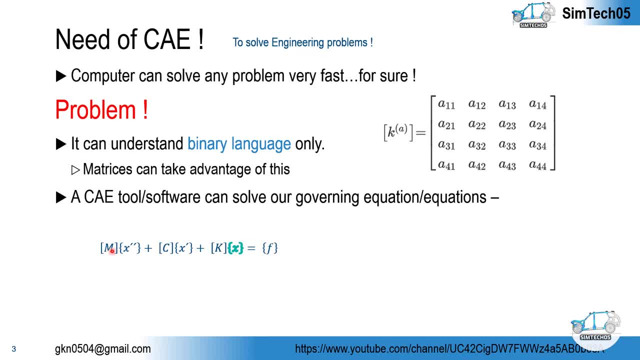 see here i represented m as a matrix, C as a matrix, K as a matrix, and these are the vectors. these equations not look like same in the numerical technique, in numerical technique, in numerical methods. these equations look like same in numerical technique, in numerical methods. these equations look like some. 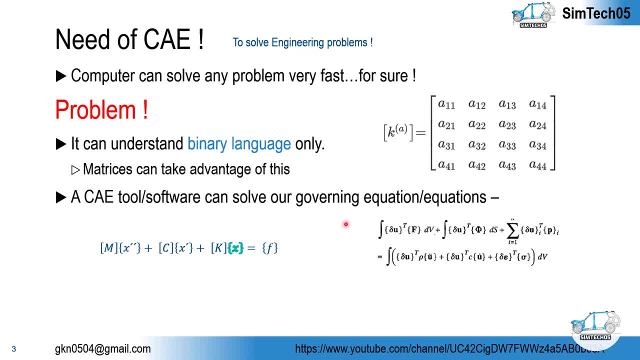 something different. actually, this is nothing but expansion of this form. So there we have two major questions. if we have any engineering problem and we want to solve that engineering problem with the help of computer, we have to convert that problem in form of matrix. So question is how we can convert our governing equations in form of matrix. 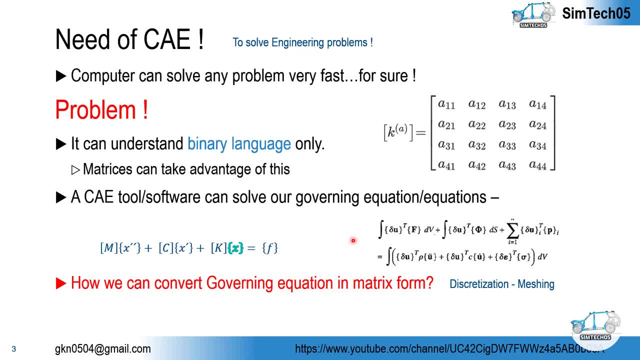 And answer is: with the help of discretization, or in other word we can say by the mashing, The discretization, not only the way. okay, after discretization, we have some methods to convert our governing equation in form of matrix. we will talk little bit about that. 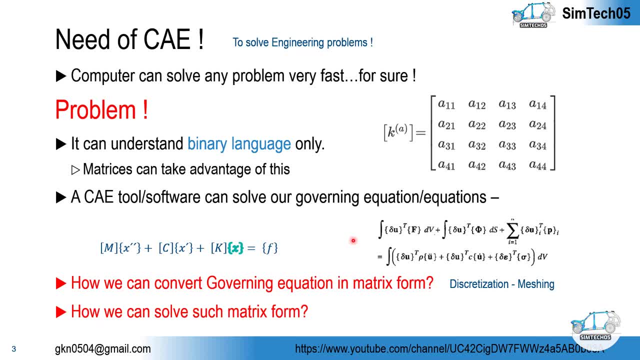 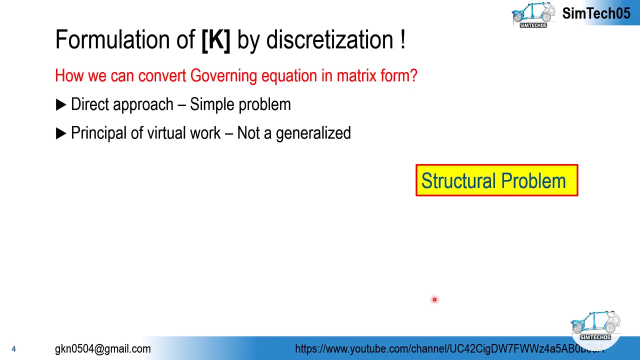 And once we have those governing equations in form of matrix, how we can solve those equations, Matrix forms? the answer is numerical methods. So now we will talk little bit about the discretization and converting a governing equation into matrix form. This we can do with the help of simple approach, principle of virtual work and related to method. 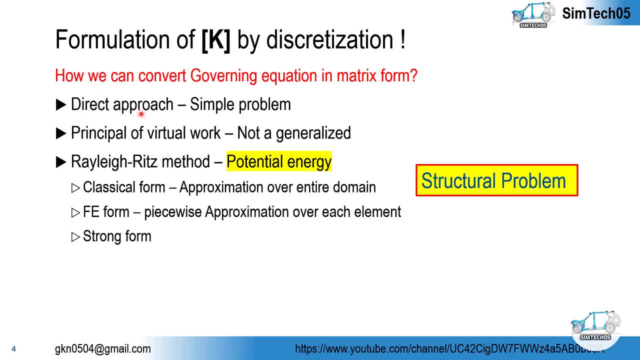 But there is problem with the simple or direct approach. Approach is applicable only for very simple type of problems. See, once we match the component, we have small small particles, small small elements and with the help of those elements we are actually converting irregular shapes into regular shapes. 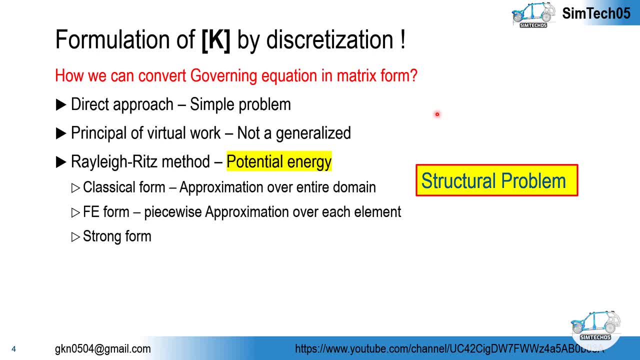 And we are locally approximating the original complex equation at the elemental level. Earlier we have governing equations. Now we have governing equation for the complete component. that may not applicable for the arbitrary structure, But for the small regular pieces we can locally approximate the original complex equation. 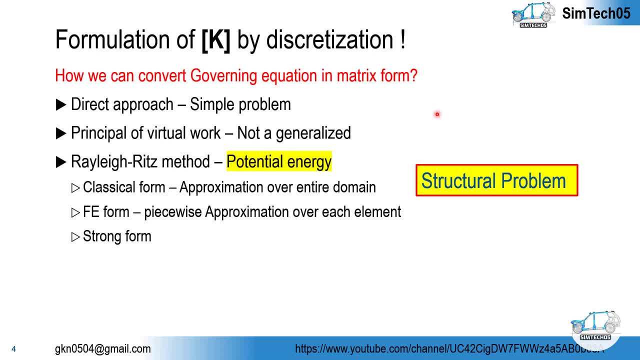 at the element level. So we may have multiple elements, we may have thousand or lakhs elements within our model. So finally, we will get a set of equations And these equations may be Algebraic Set of equations, Ordinary differential equation, or may be partial differential equation. that depend on our problem. 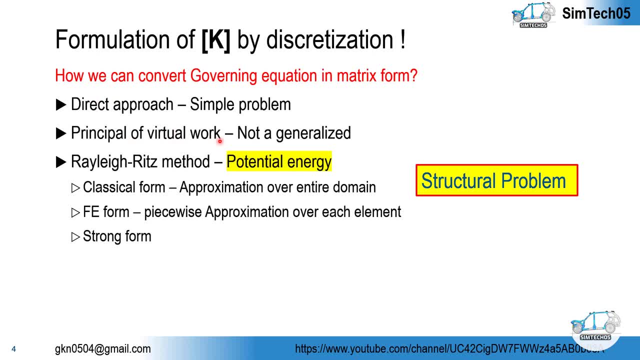 So again, the direct approach, principle of virtual work method. those methods or related method convert and governing equation in form of matrix equation. The mathematics behind those methods are not that much easy, But once you familiar with these methods you can form the stiffness, matrix and integral. 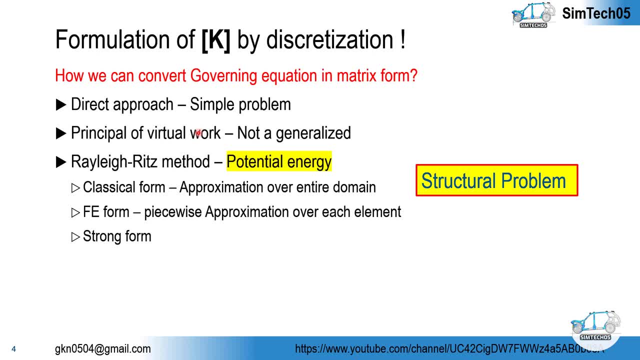 form of governing equation for the simple problem manually, and for complex problem you may need to utilize some programming tool like MATLAB. Okay, If you want to learn more about these approaches mathematically a generalized governing equation into form of matrix and how they can find. 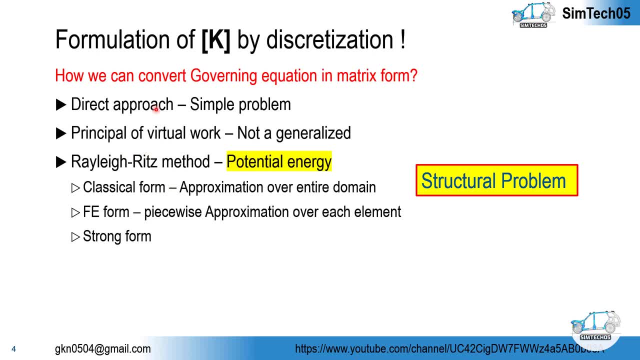 Or how we can find the stiffness matrix, Mathematically, A generalized governing equation into form of matrix and how they can find, or how we can find the stiffness matrix. With the help of these approaches you can follow the NPTEL lectures And related method is: 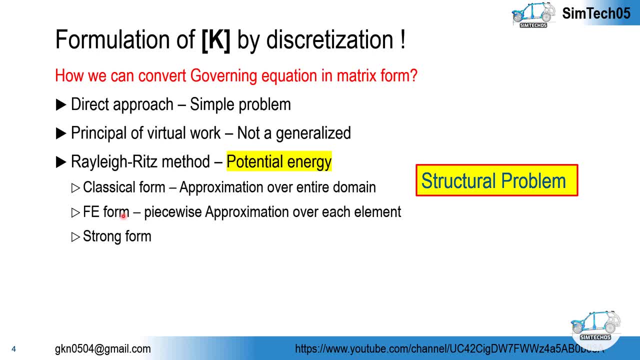 Having two way. One is classical form and one is EFI form. And good thing. the related method is strong form. You may listened about those strong form. They're strong form where we have differential equation plus boundary conditions for the functional and weak form. only we have differential equation for the functional. 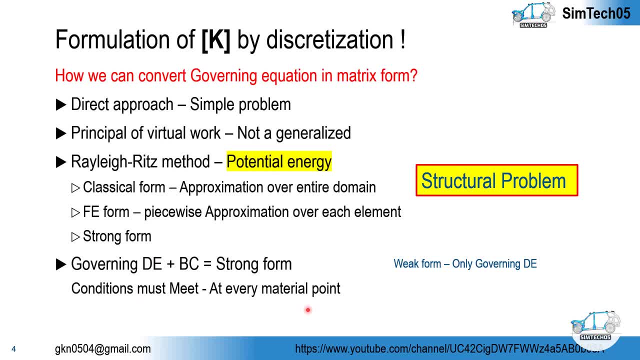 In the strong form the condition meet at every point within the solution space, or we can say at every material point. and in the weak form these conditions need to meet only in the sense of average form not necessary to meet the material point. material conditions at each and every point. 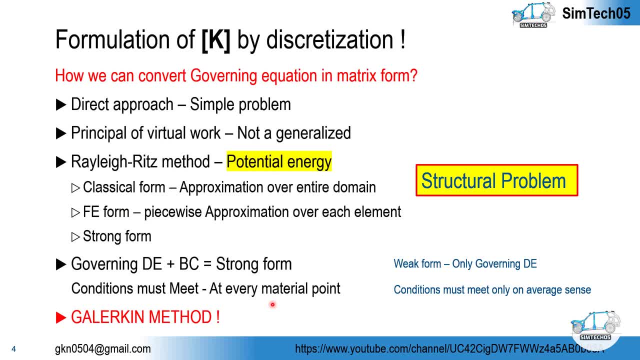 You may listen. one more technique. you may heard about that: Galerkin method. If Rayleigh Ritz method is based on potential energy approach- and it's a strong form, then why this Galerkin method is exist As suggested by Robert D Cook finite element book. 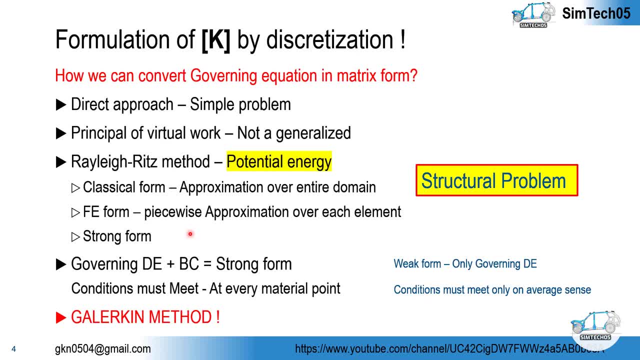 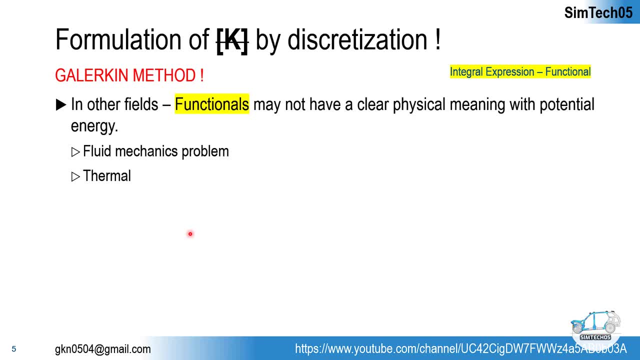 This Rayleigh Ritz method is very acceptable for the structural problem because in the structural problems the functional Functional is nothing but integral expression or integral statement, ok, nothing else. So I am saying functional In the structural problem, this functional having a physical meaning with respect to 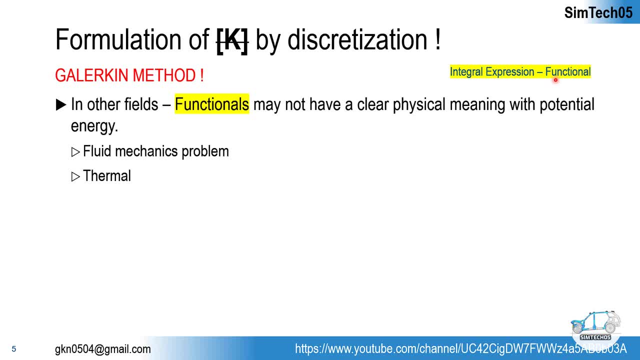 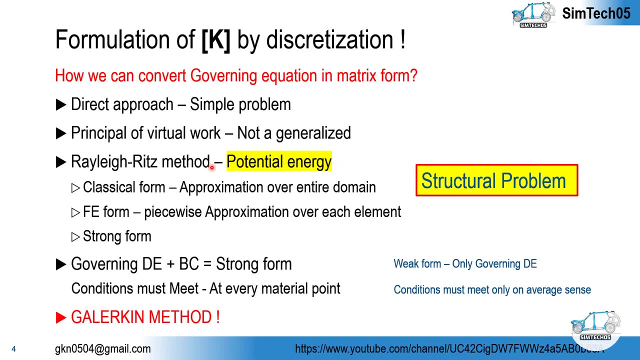 the potential energy But in many cases, especially in term of Thermal problems or maybe fluid mechanics problem, These functional may not have clear physical meaning with the potential energy. Why we are talking about potential energy, if you remember, the Rayleigh Ritz method based. 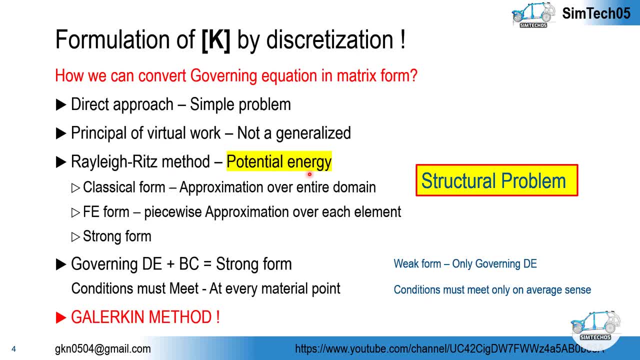 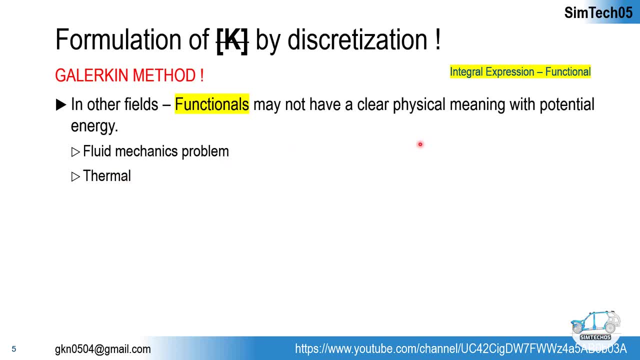 on the potential energy method And this potential energy may not having a physical meaning with respect to thermal problem, fluid dynamics problem and such problems. That's why, Apart from the Structural problem, people start looking to other method, And this is nothing but your Galerkin method, based on the weighted residual scheme. 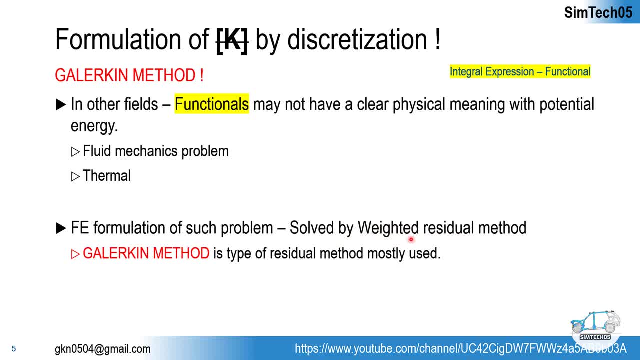 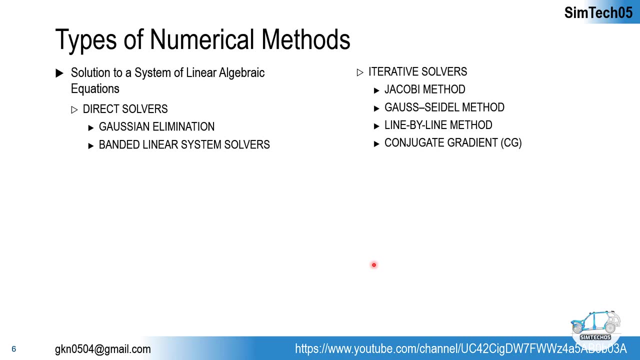 Of course, we have multiple methods in the weighted residual scheme and Galerkin is the one of the widely used method due to its advantages, Once you know how to Convert a general equation into form of matrix, or you can say with the help of discretization, 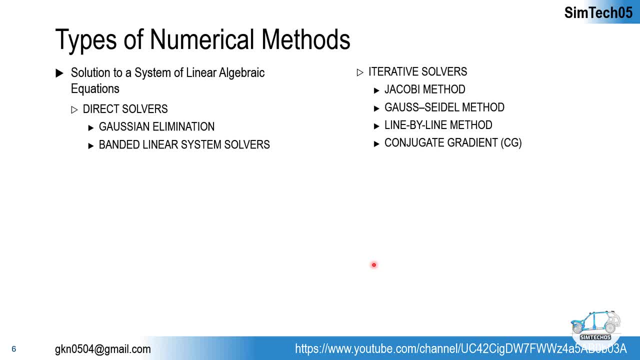 once you locally approximated the original complex equation at the element level And you have a set of equations, Then the second question arises: how to solve those set of equations. and these set of equations can be solved by the different numerical methods. Let's see. 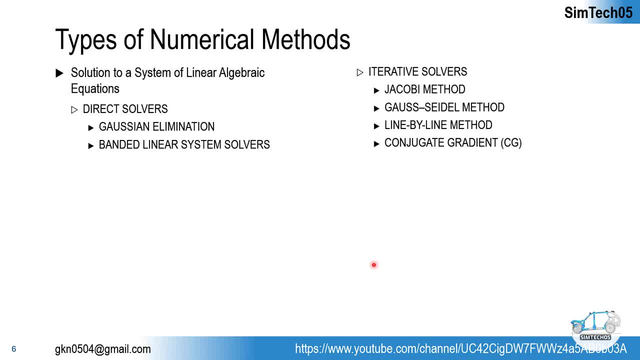 Let's see, And it depends what type of setting set of equations you got. if you got linear algebraic equations, you have to approach direct solvers. you have iterative solver, you have. See, if those set of equations are linear algebraic equation, then we can solve it very easily. 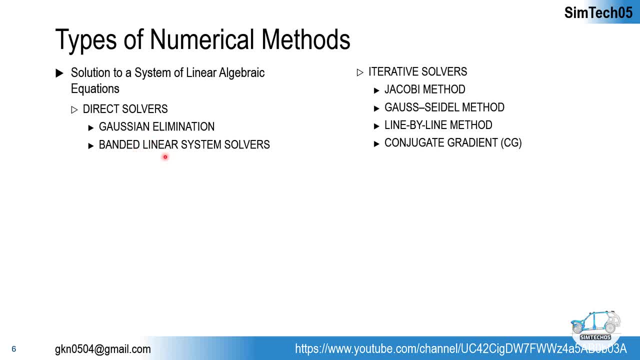 OK, those Gauss elimination method and banded linear system solvers in iterative Jacobi-Gauss system solvers And conjugate gradient method, line by line method, those all methods are available. But if you have set of equation in term of ordinary differential equation, 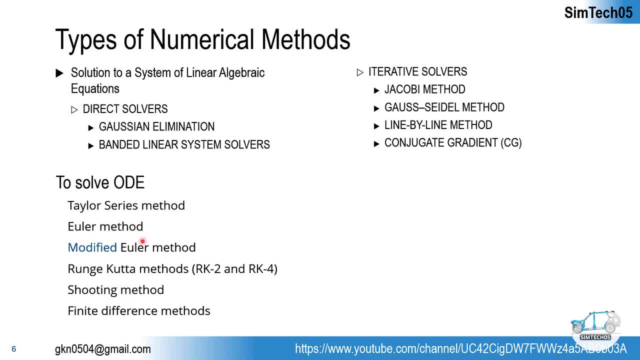 Then these are the different methods: Euler method, Taylor series method and those all methods. And if you have partial differential equations, set of partial differential equations, then we have to utilize the finite difference. finite element method, finite element method, finite point and volume method may be mess. less technique, multiple method, etc. 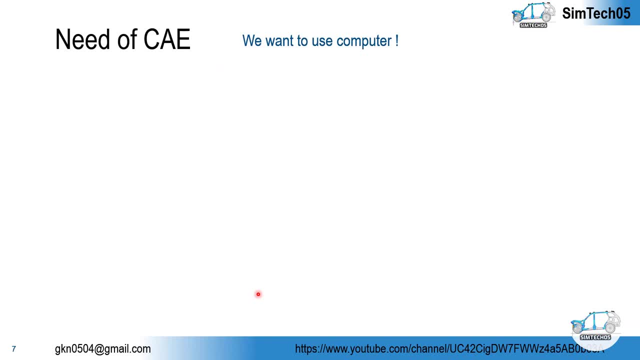 So again to summarize, I need to solve an engineering problem with the help of computer, added engineering, and we want to utilize the computer. and for that engineering problem we have ordinary differential equation or partial differential equation with the space variable and boundary conditions. If those ordinary differential equation and partial differential equations are quite easy, 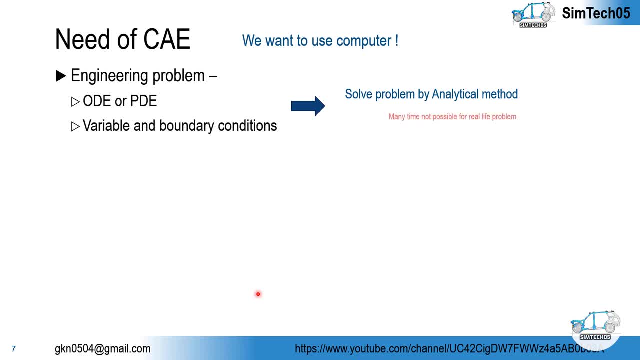 then we can solve them directly by analytical method. OK, but many time it is not possible in real life problem Because the problem become very complex. So what we have to do that time? we are going to discretize our problem and we are going to convert, or we are going to approximate the original complex equation. 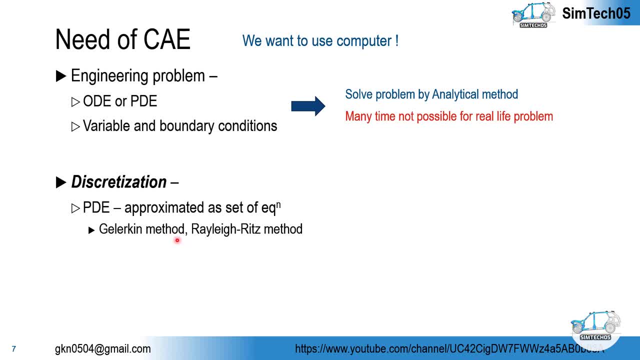 With element level, and for that we have different methods, like Rayleigh rates method and Galerkin method, etc. So this is the example. this outer boundary, that red boundary, is representing an arbitrary shape, and we can discretize that arbitrary shape into small, small regular triangle shapes. 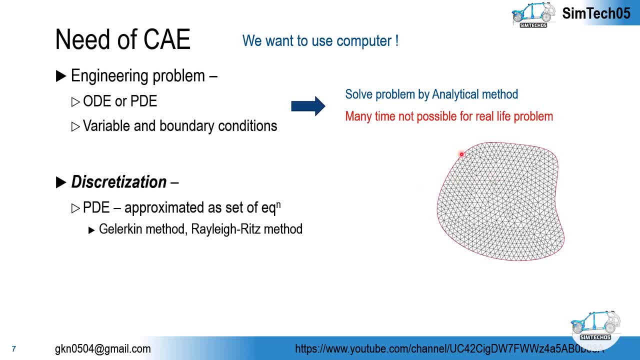 We may not able to approximate this arbitrary shape by help of the governing equation, So we can use this example. So we can use this example. So we can use this example. We can use this example by see governing equations, but we can approximate the governing. 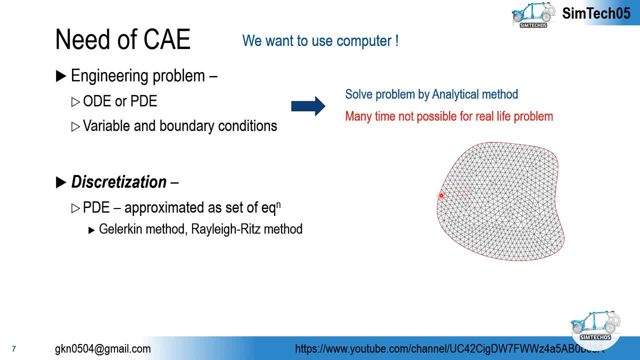 equation at the element level. So converting this domain into a small, small domain is discretization, and with the help of this discretization We are finding the set of equations, and those set of equations form a metric equation with the help of Galerkin, Rayleigh, rates method or any other method. 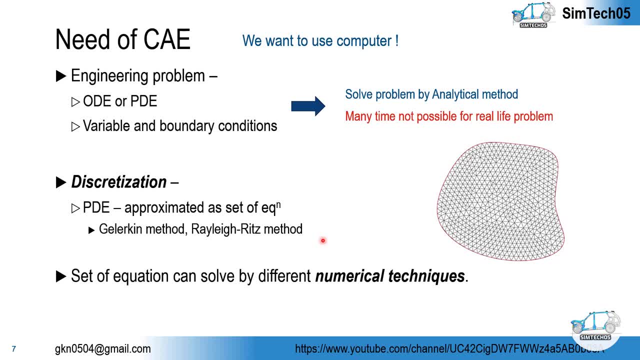 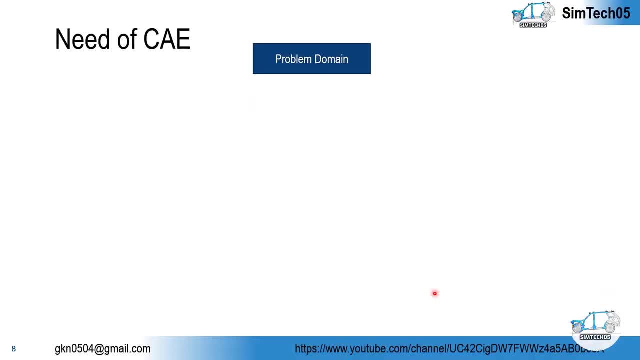 And So solve final matrix equations, we have to utilize the numerical techniques. so again, I represented the whole discussion in form of flowchart. if we have problem domain, of course we can generate some analytical algebraic equations or partial differential equation, ordinary differential equations for the problem. 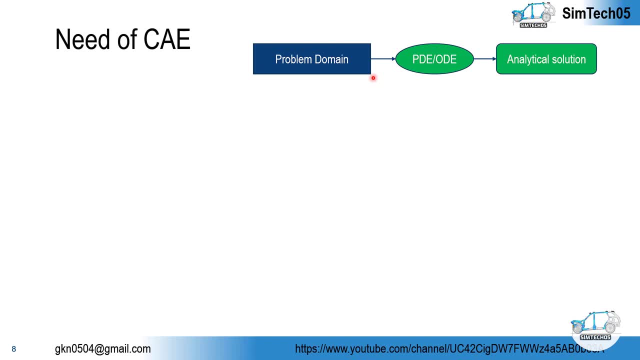 like someone, provide the growth factor in the Y with respect to X. we can organize them as per the given boundary conditions and we can generate a algebraic equation for that. similarly, we can generate partial differential equation or ordinary differential equation, depend on the problem statement. of course we have your space variable and boundary conditions, but if those 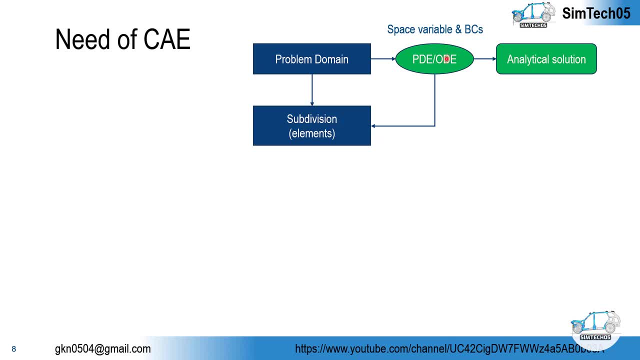 equations are not very easy to solve, then we can use the problem statement to solve the problem. easily to solve for the particular domain means our domain is very arbitrary, it's not a regular domain, then we have to subdivide it, we have to discretize the domain and we have to convert the domain into small, small particles. those 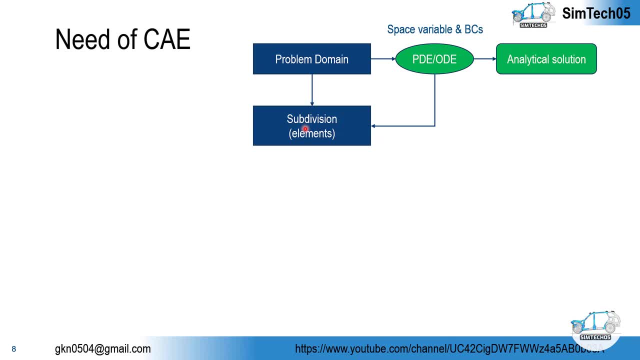 particles are called element. and why we are doing this? because we want a regular shape on which we can apply the governing equation. so again, for that we are locally approximating the original complex equation at the element level. so once we done with it, discretization- see, we have discretization and after that we will get the element. 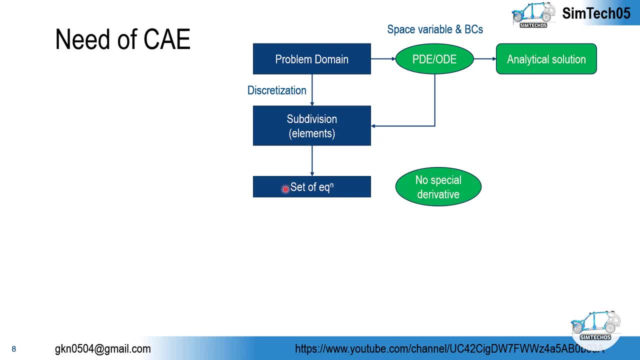 so after subdivision we will get set of equations earlier. we may have special derivative that may not able to, that we may not able to solve very easily, but right now we don't have special derivative which is very difficult to solve, as long as we can get that element. 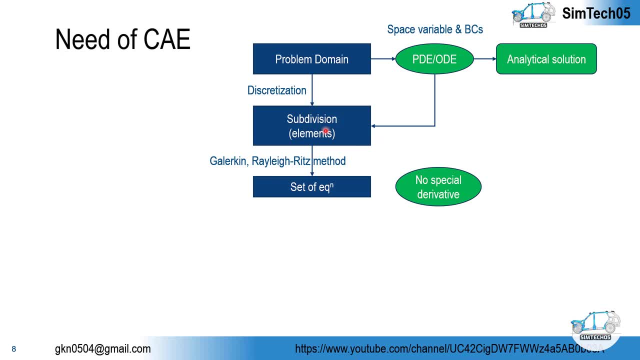 don't have such any special derivative, and this we can do with the help of subdivision. we can find out the set of equations with Galerkin or Rayleigh Ritz method. see, I am taking here only two name. it's not been only those two methods. you can utilize number of 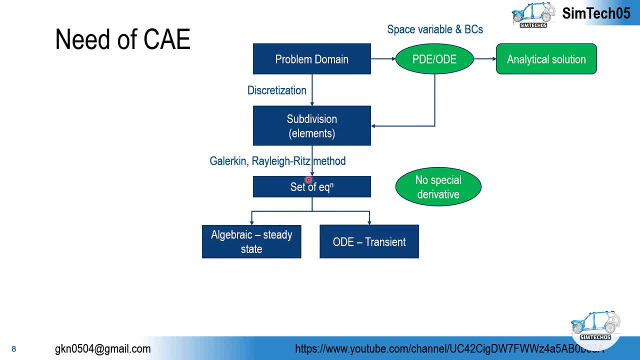 methods for the same and once you have set of equations, we have to solve them. if those are the algebraic equations, we have different method. if they have ordinary differential equation or partial differential equation, we have different method. in general way, if the problem is a steady state problem, we will get the algebraic set of equation, and if the 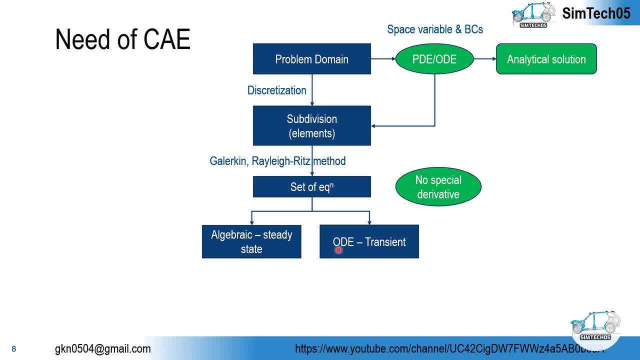 problem is transient problem. we will get the ordinary differential equation set and just for example, again Gauss-Linemason method you can utilize here and here Euler method or another method you can utilize, and these things we not need to do manually. computer take care of these. all things. of course, subdivision, discretization, we have to do manually. but 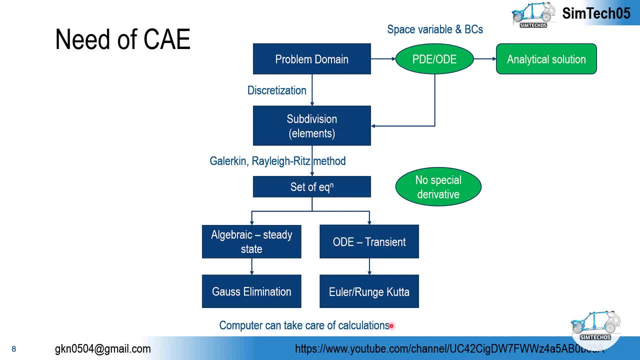 now days, discretization also automated. so here we have an example for the Gauss-Linemason method. of course, you may able to find this Gauss-Linemason method very easily. I always saw this method in my previous videos. So just to utilize the NPTEL lectures, this example taken from practical finite element. 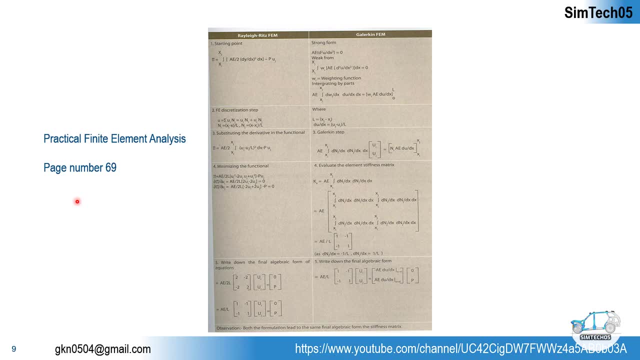 analysis book by Nitin Gokulisar, in page number 69. so very simple bar element is taken and for the bar element both Euler's and Galerkin method applied and finally the stiffness matrix is written, as well as the complete equation in form of matrix is written. 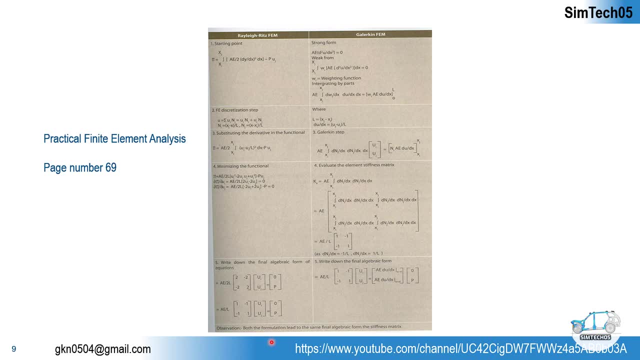 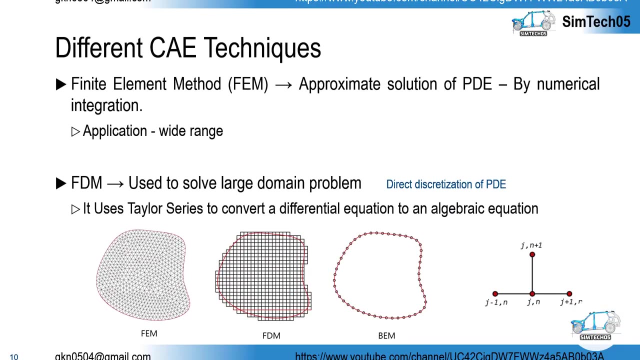 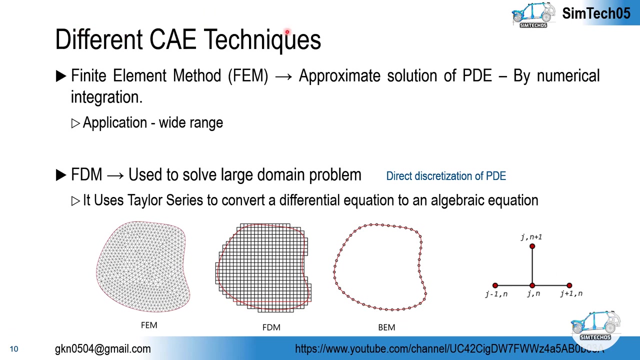 That we can solve with the help of manual methods or computer. okay, there should be numerical, different numerical techniques to solve any problem. so of course we have finite element method that approximate the solution of partial differential equation by numerical integration approach, And wide range of application is available for that within the one figure you are able. 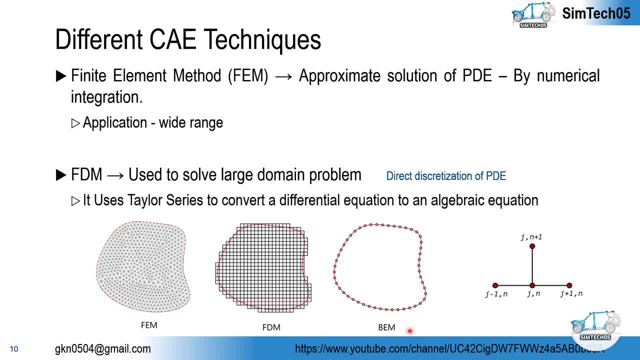 to understand the difference between FEM, FDM and bound element method. FEM is quite common approach to solve any arbitrary shape, but FDM is limited to regular shapes because FDM utilize the difference method In the solution on the nearby point with the help of gridding scheme. so that's why the regular 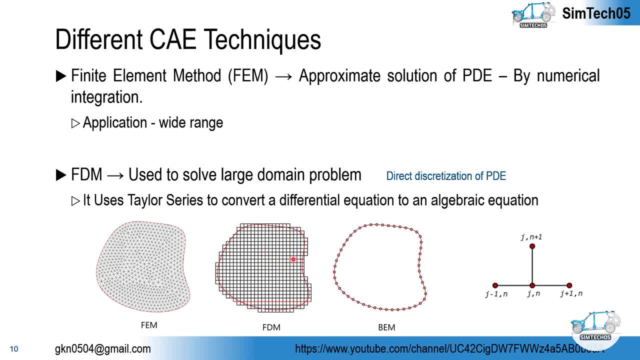 matching is very important for the FDM procedure And the boundary element method is utilized when you are interested to see result only on the boundary of the outer boundary of the domain. you are not interested within the domain. what happening within the domain, it's not important for you, and finite volume method.